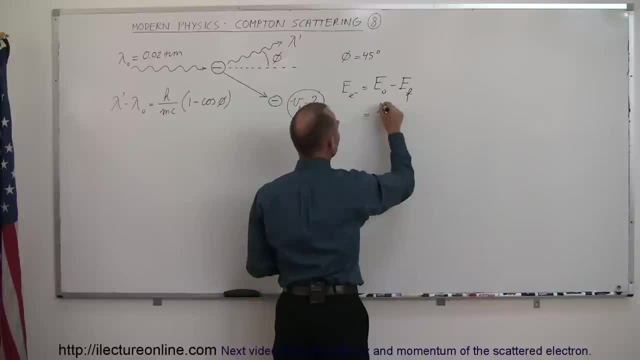 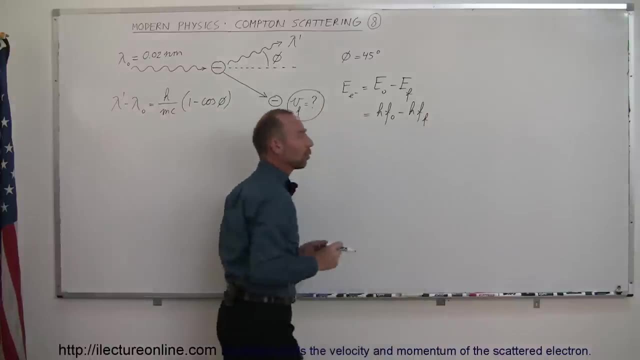 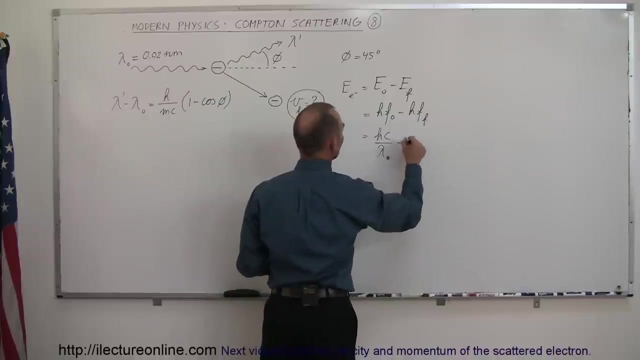 And how do we find the energy of the photon? Well, the energy of the photon is equal to h times the original frequency minus h times the final frequency. And of course the frequency can be written as c over lambda, so this can be written as hc over the original lambda minus hc over the final lambda, And of course we have the final lambda as lambda prime in our equation. 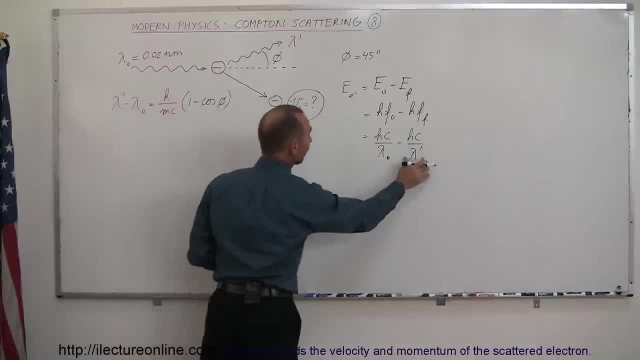 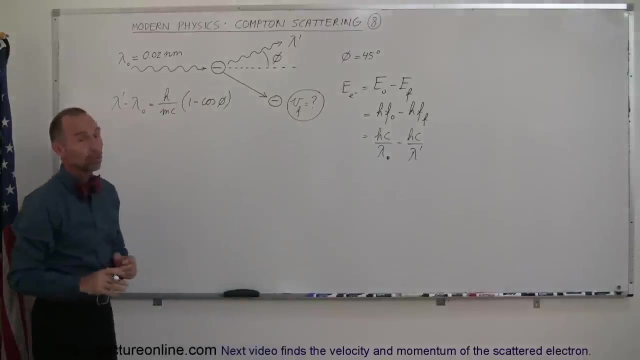 Okay, so all we have to do is find the final wavelength plug in the initial wavelength here. Here's the difference in the energies, That will be the energy given to the electron. Okay, so we see the strategy here. So next we're going to solve for lambda prime. So lambda prime is equal to- I move this across- lambda initial plus h, over mc times 1, minus the cosine of phi Plug. in the numbers that we have This here would be equal to 2 times 10, to the minus 11 meters plus h, which is 6.6.. 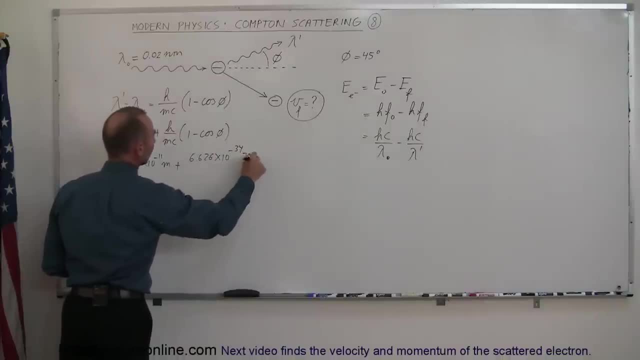 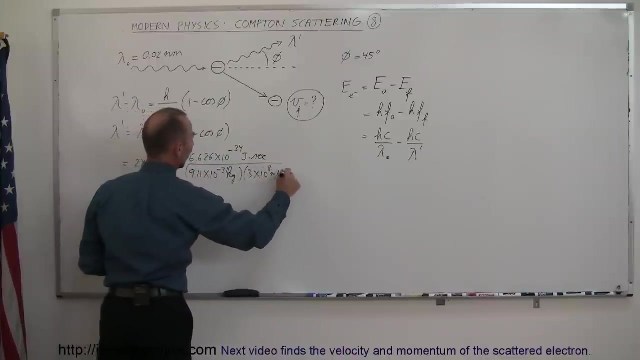 6.6 times 10 to the minus 34 joules times seconds divided by the mass of an electron, 9.11 times 10 to the minus 31 kilograms. And we multiply that times the speed of light, 3 times 10 to the 8 meters per second. And then we multiply that times 1 minus the cosine of 45 degrees, which of course is 0.707.. 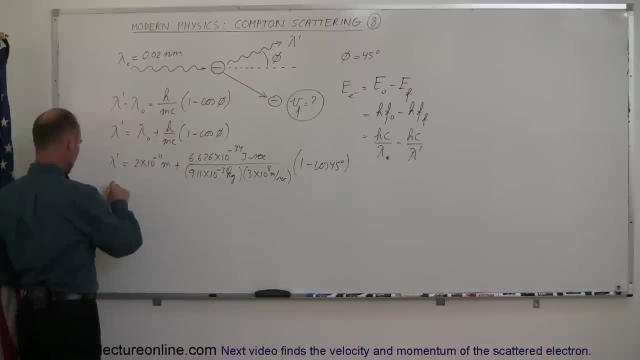 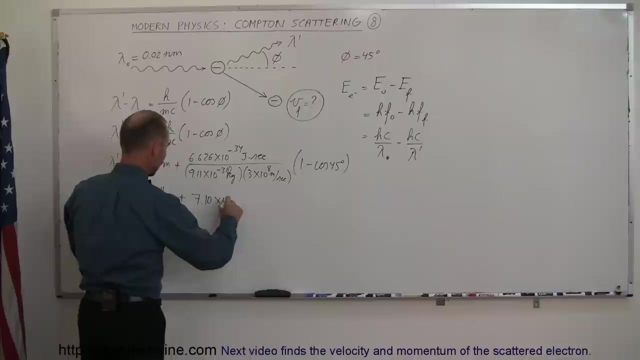 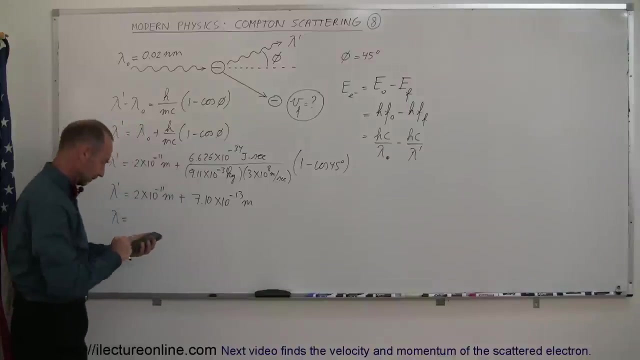 Okay, so that means the new wavelength of the electron is equal to 2 times 10 to the minus 11 meters, plus change, And so that would be 7.10 times 10 to the minus 13 meters. So if we add those two together, what do we get? So it'd be 2.071 times 10 to the minus 11 meters. All right, so that's the new wavelength of the electron. 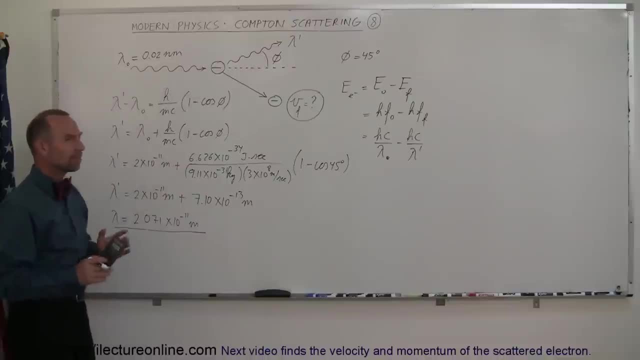 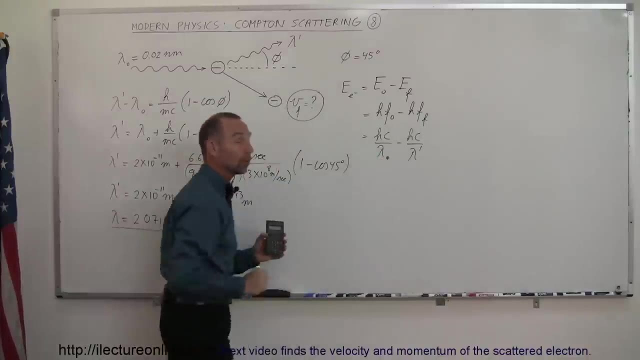 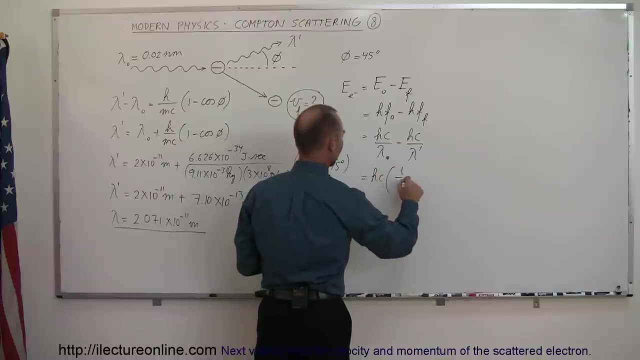 the photon after it scatters off the electron. Here's the old wavelength. That means it's lost some energy, And we can calculate the difference in the energy now that we know the initial wavelength and the final wavelength using that equation right there. So that's going to be equal to- let's factor out an hc hc times 1 over lambda initial minus 1 over lambda final. Okay, so Planck's constant 6.626 times 10 to the minus 34 joules times seconds. 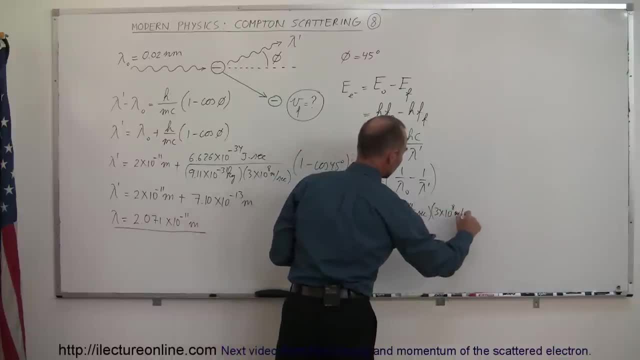 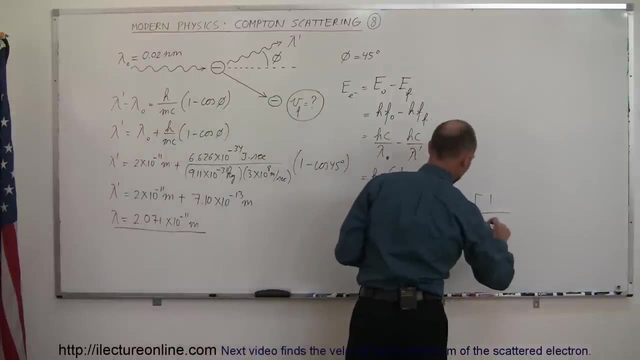 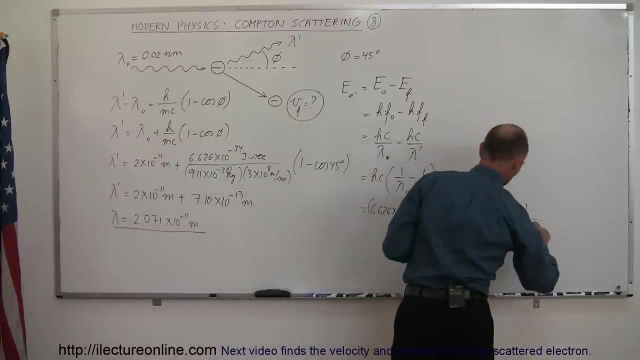 Speed of light: 3 times 10 to the 8 meters per second, times 1 over the original wavelength, which is 2 times 10 to the minus 11 meters, minus 1 over the final wavelength, which is right there: 2.071 times 10 to the minus 11 meters. 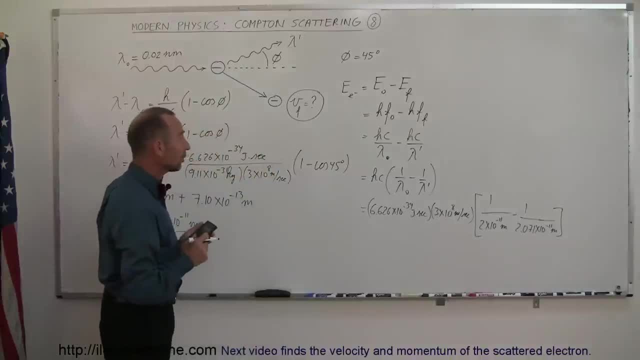 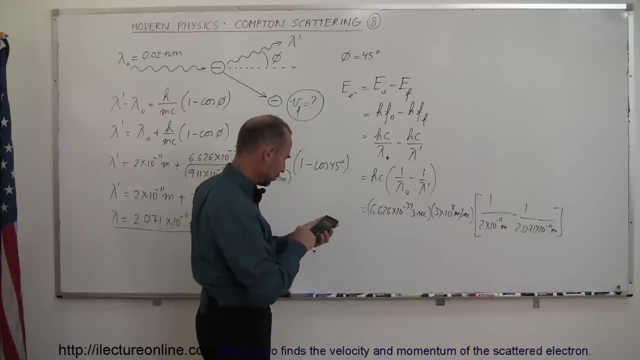 And that will give us a change in the energy of the photon, which means that's the energy imparted on the electron. All right, So 1 divided by 2e to the 11 minus minus, 1 divided by 2.071 e to the 11 minus equals- Ah, that's a lot better. And we multiply the times 3e to the 8 and times 6.626 e to the 34 minus, And here we go. 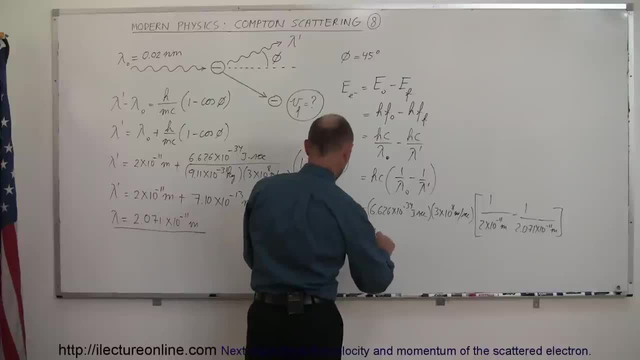 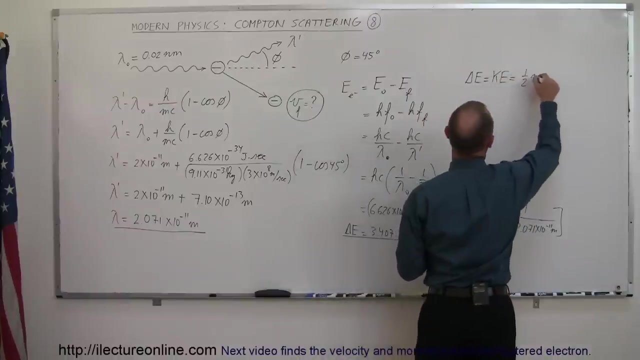 So the difference in the energy is 3.407 times 10.. That's the change in the energy, and that would be the energy given, of course, to the electron. Now, that would be kinetic energy. So the change in the energy in the photons equals to the kinetic energy of the electron, which is equal to 1 half mv squared. 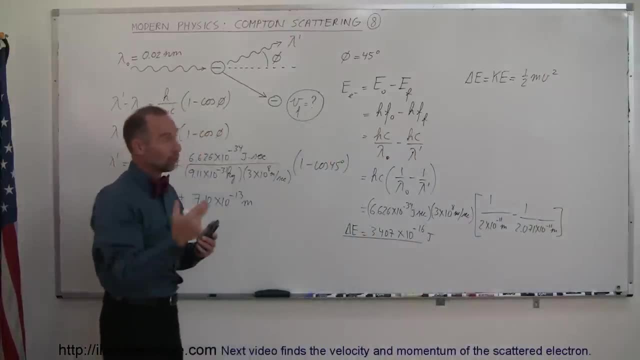 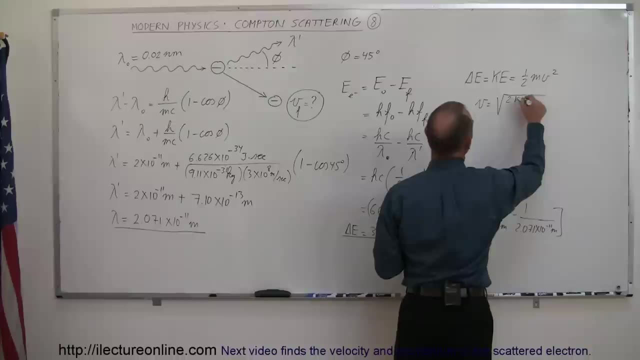 And ultimately we're trying to find the velocity of this electron. So, using that energy, let's find the velocity. So the velocity is equal to the square root of 2 times the kinetic energy Divided by the mass of the electron. 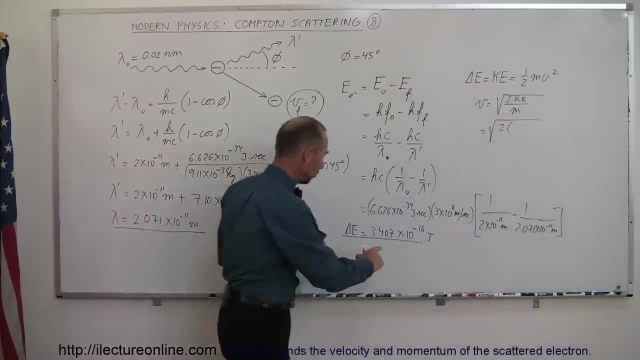 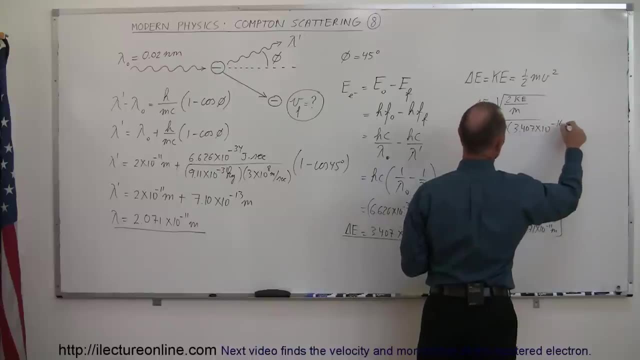 So the square root of 2 times the kinetic energy that we just found, which is 3.407 times 10 to the minus 16 joules, And divide the whole thing by the mass of an electron, 9.11 times 10 to the minus 31 kilograms. 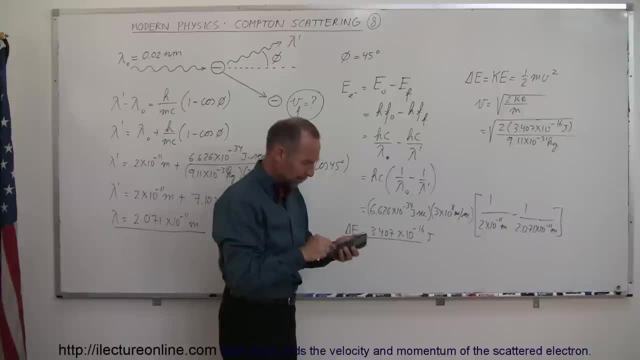 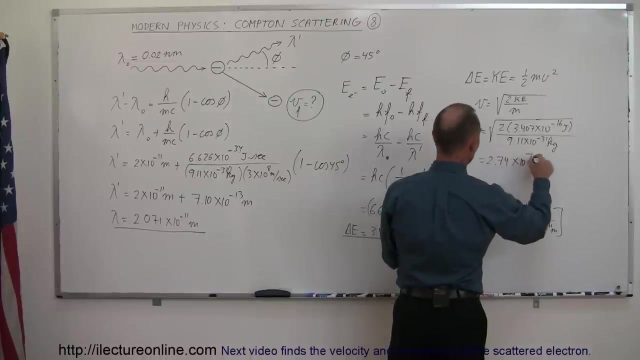 Okay, So divide by 9.11 e to the 31 minus equals Equals, and then times times 2 equals. and now we take the square root of that and there we go. So it's equal to 2.74 times 10 to the 7th meters per second. 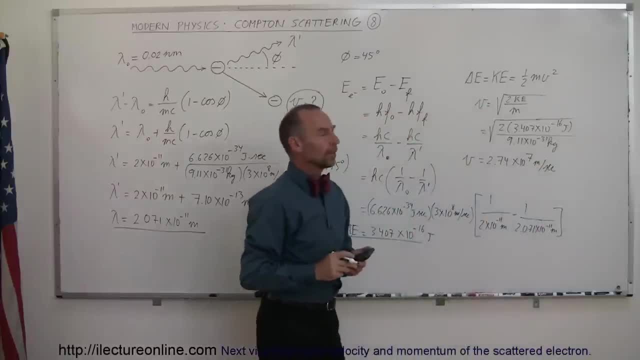 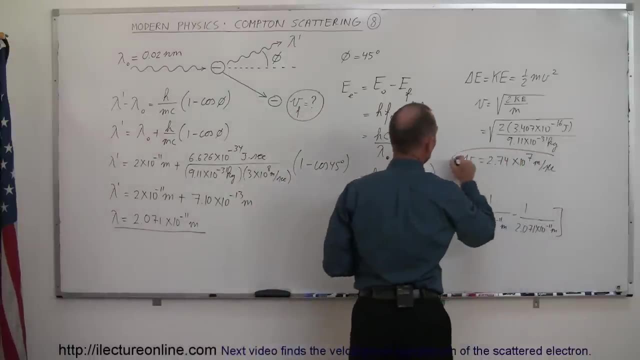 Wow, that's quite fast, Because that's almost 10% of the speed of light, because speed of light is 3 times 10 to the 8 meters per second. However, since it's less than 10%, we can assume that to be somewhat non-relativistic. 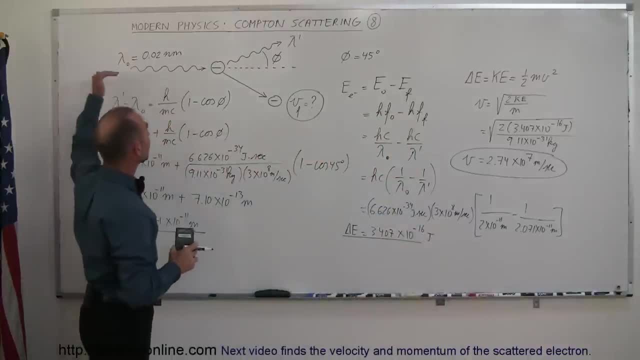 And so this electron, having been hit by a photon of this wavelength, would have gained a speed of almost 10% of the speed of light, after that photon scattered off of it with an angle of 45 degrees, And that's how you use the Compton scattering to figure out the velocity of an electron that's been hit by a high energy photon. Okay. 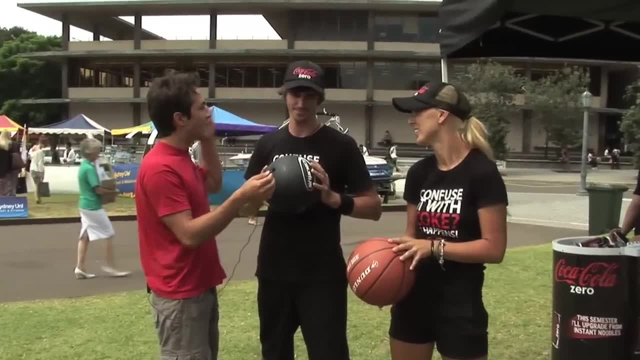 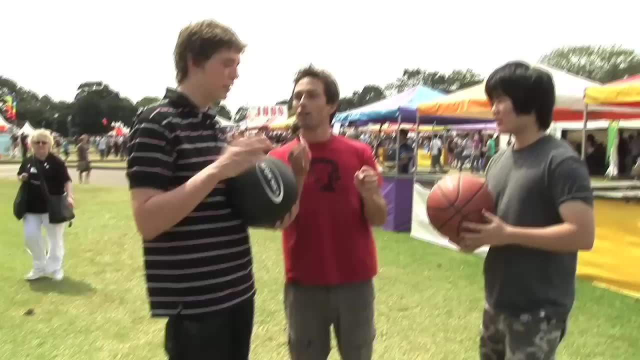 Let's say, a Jack holds both balls above his head and then he drops them at exactly the same time. What do you expect to see? Well, they're gonna hit the ground at the same time. I expect them to both land at the same time. same time, same time. 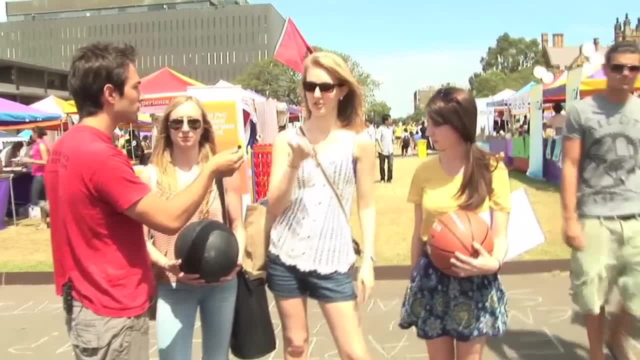 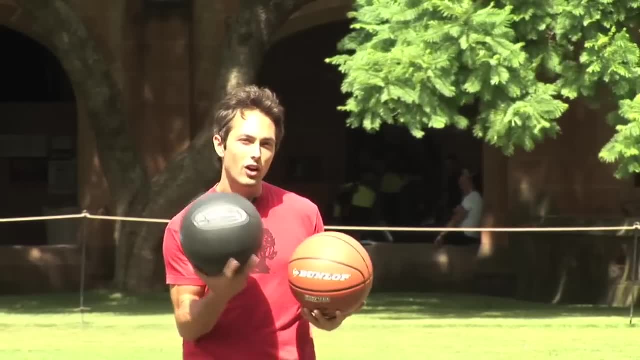 I think they both will. Well, you would expect this one to hit the ground first. However, they would actually both hit the ground at the same time. Why's that? Science, Yeah, science. Now, the black one clearly feels a lot heavier. 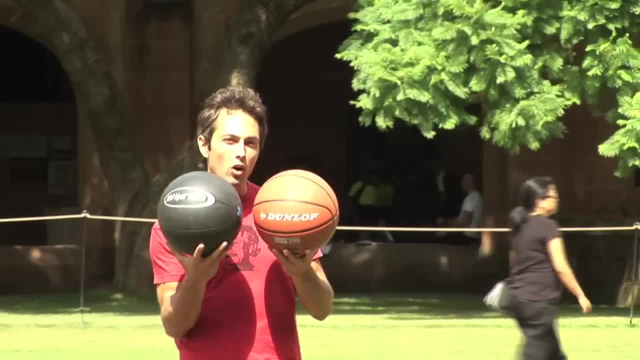 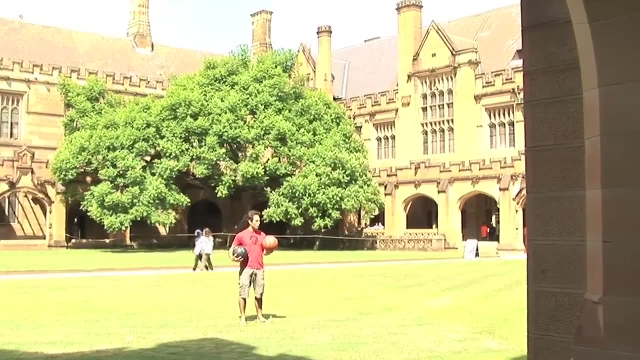 So the standard misconception is to believe that the black ball will accelerate at a greater rate and reach the ground first. This year, many people had an idea that both balls would land at the same time, but they didn't know exactly why. I found there were some different misconceptions. 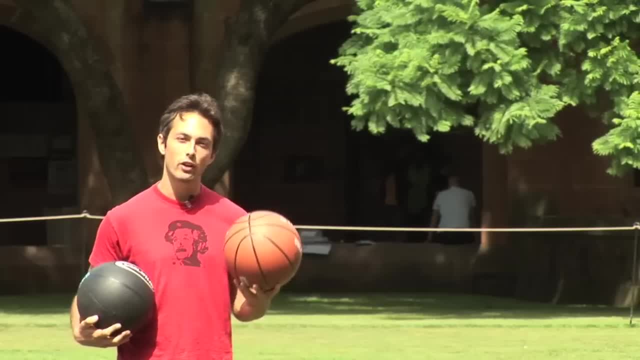 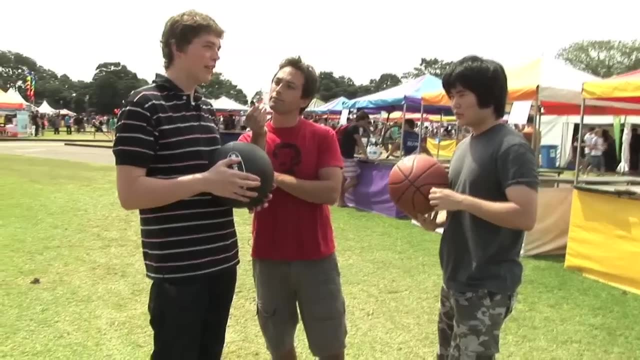 For example, many people seem to think that as an object falls towards the earth, it falls with a constant speed. From this height: yeah, pretty much Just a constant speed. all the way down speed: Yeah, I think it would be the same constant speed. 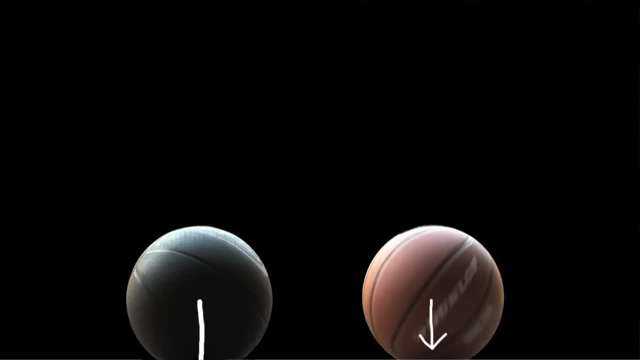 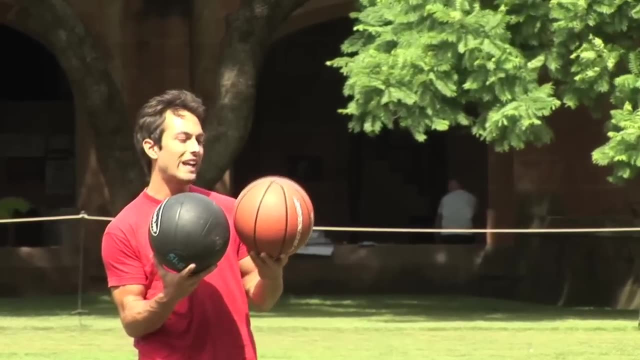 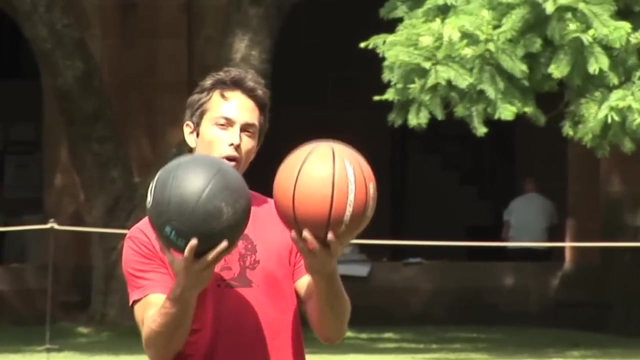 It makes them accelerate, It gets them to speed up. Another misconception I discovered was that some people believe both balls should have the same gravitational force on them, even though the black ball is clearly much, much heavier. The reason I think they said this was because they knew both balls needed to reach the ground at the same time.